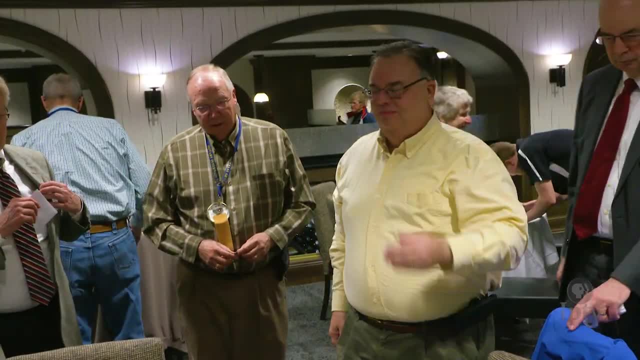 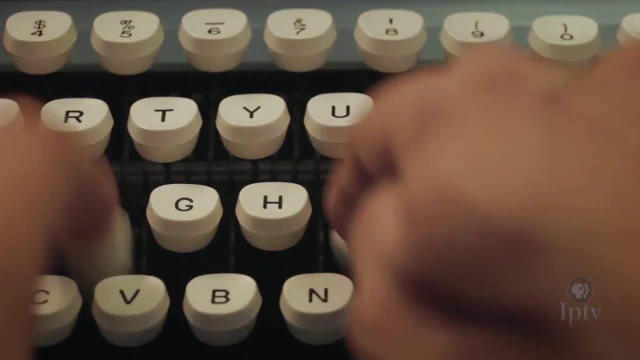 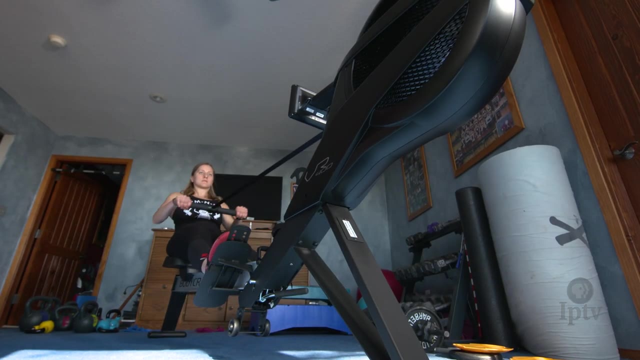 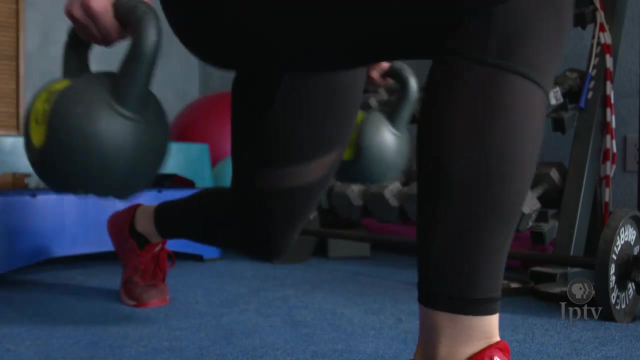 You have to take no a lot or, in my case, you have to endure really disgusted faces. People who are active definitely need to get a little extra protein in their day-to-day basis. just from a recovery, I was able to get a little extra protein in my day-to-day basis. from a muscle building standpoint, 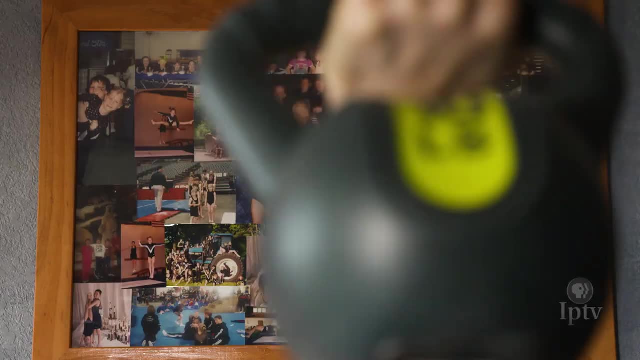 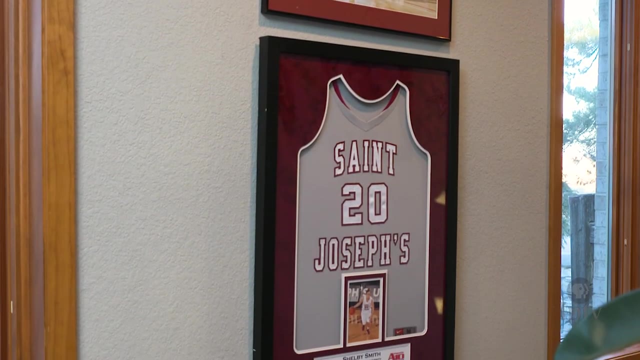 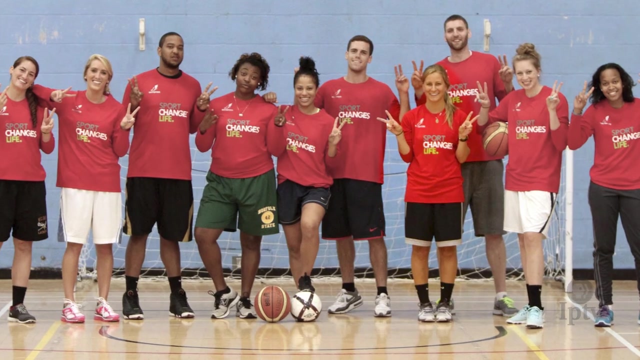 So for me that was one of the main draws to get into insect protein. I grew up playing all sorts of sports, ended up landing on basketball, Was lucky enough to earn a full scholarship to St Joseph's University out in Philadelphia, and then was again lucky enough to continue my career in Ireland as part of a program called 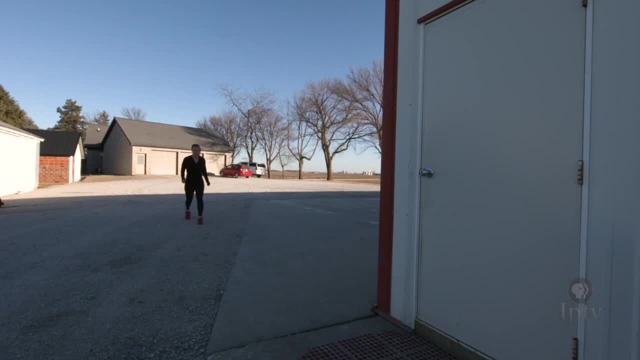 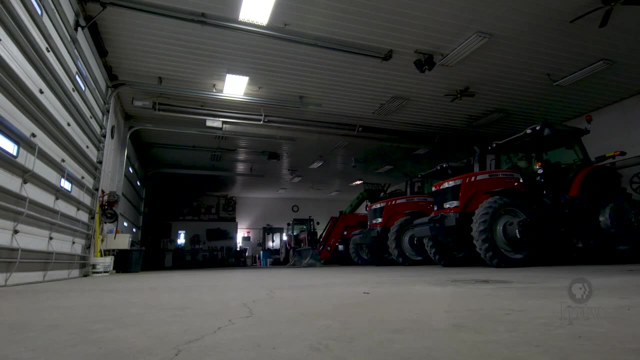 Sport Changes Life. I graduated with an MSc in Finance from Trinity College in Dublin. I went into the finance industry and I actually found myself really unhappy. Moved back here to Iowa to see if I could try my hand at farming with my dad. 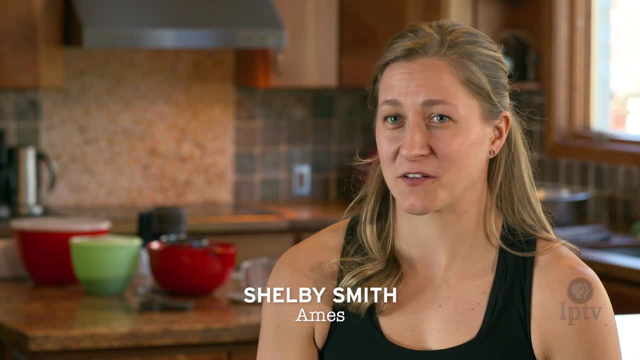 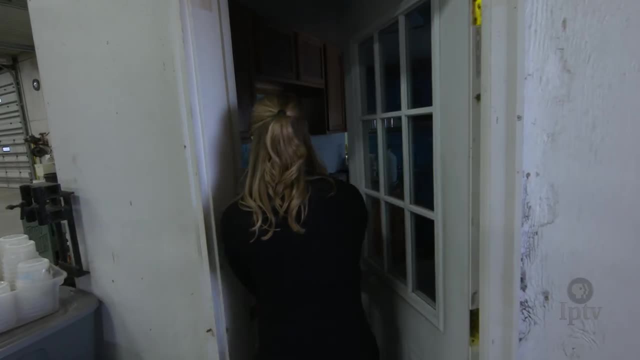 I got back didn't even know how to drive the tractor. so day one learned how to drive the tractor, day two got put in the grain cart, spilled corn everywhere, Made it through harvest, survived, and then all winter my dad encouraged me to look at other niche markets. He said 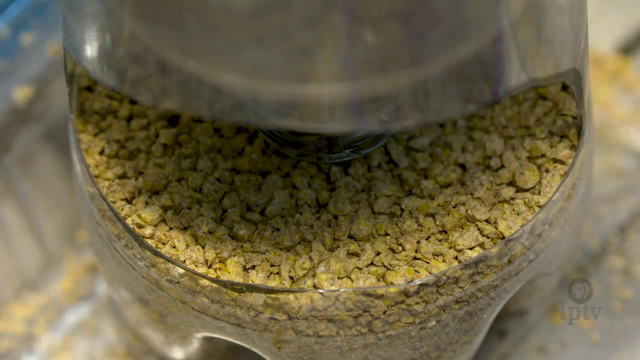 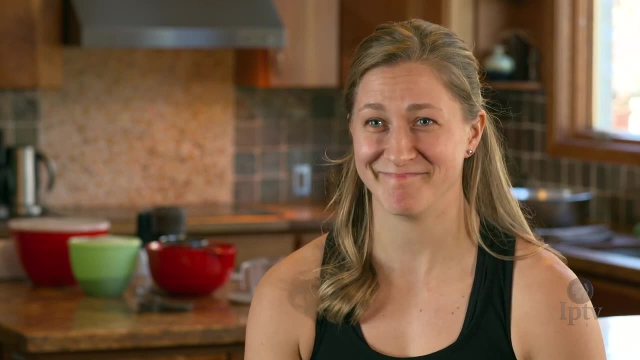 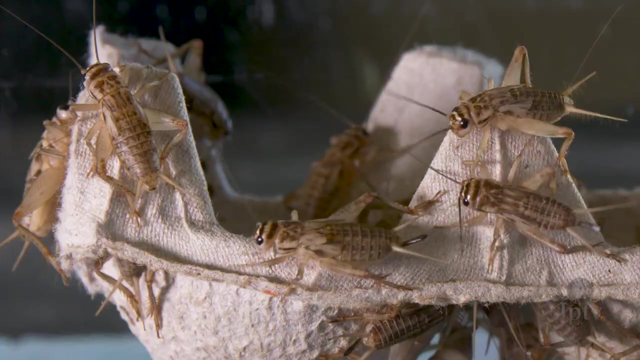 you don't have to fight the same markets I did. If you want to find a niche, go for it. We'll help you get started. So I sent them an article about raising crickets for human consumption. Crickets- people don't know it, but are actually a nutritional powerhouse. 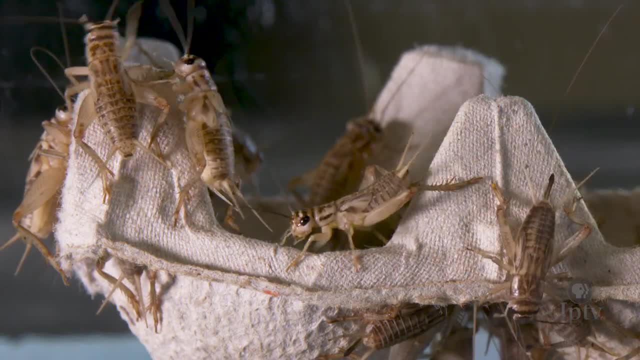 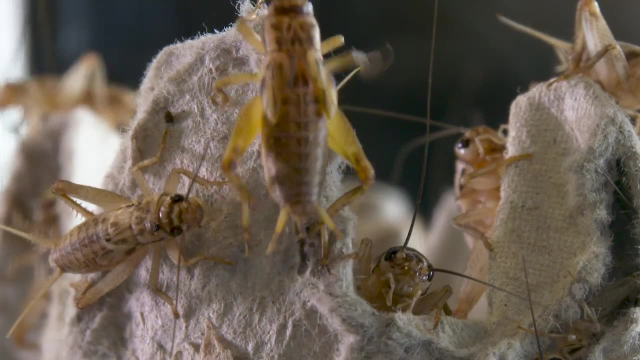 and they're also very sustainable in terms of a source of protein. They have more iron than spinach, more calcium than milk. they're a good source of vitamin B12, have a good ratio of omega-6 to omega-3 essential fatty acids. 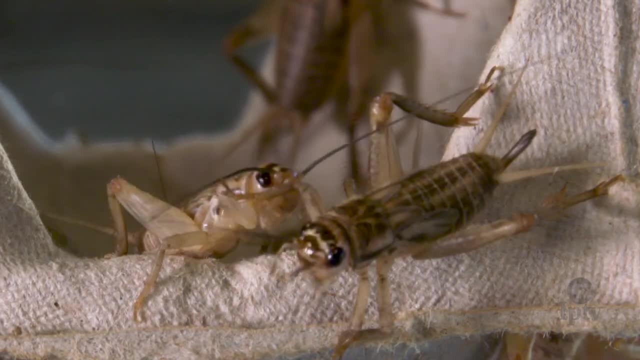 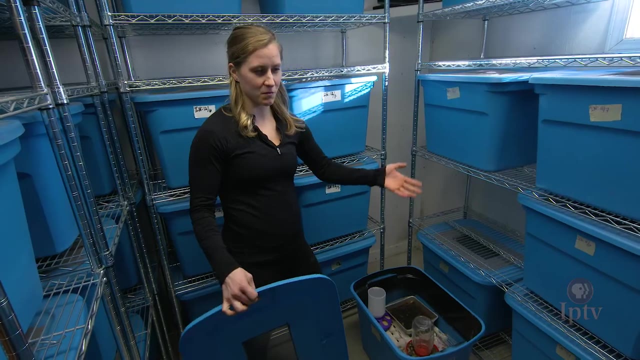 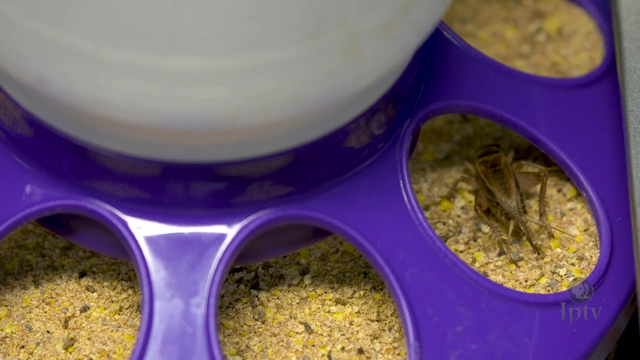 and all nine essential amino acids, so they are a complete protein. Welcome to my orchestra. That's actually what you call a group of crickets. Fun fact, I might win you a trivia contest at some stage In this room. I probably have close to a quarter million crickets. 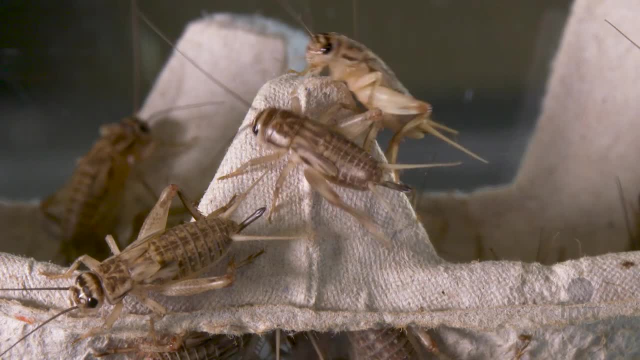 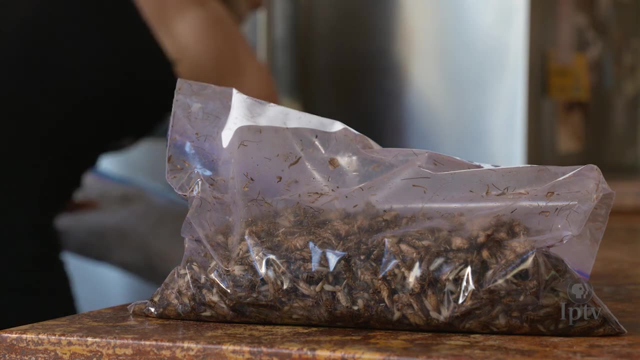 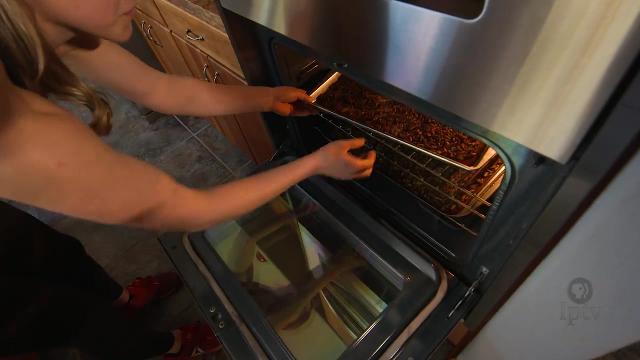 Started off with two of these blue bins. It's been an adventure For cooking. the initial step, obviously, is to kill them. They're killed in the freezer- Natural death, just like happens to every bug in Iowa. So after these guys have roasted for just about eight hours, they get pulled out of the oven. 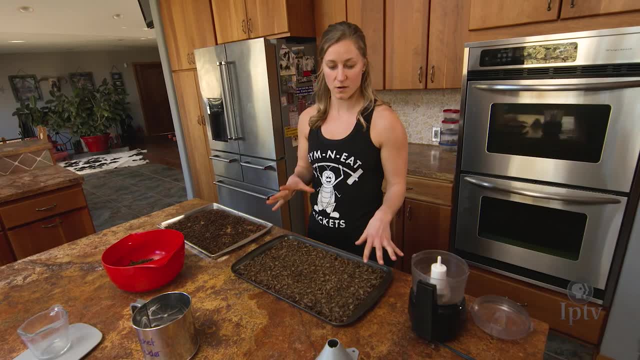 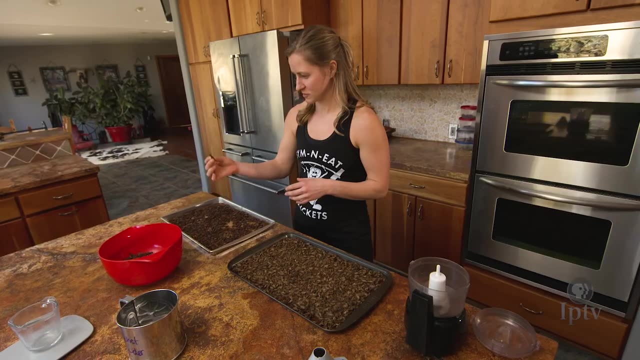 These ones right here are unseasoned, unflavored, so these will be ground into a powder. And then these ones over here. they're dry roasted, they're flavored. These ones are maple chipotle. They're just a crunchy little snack. 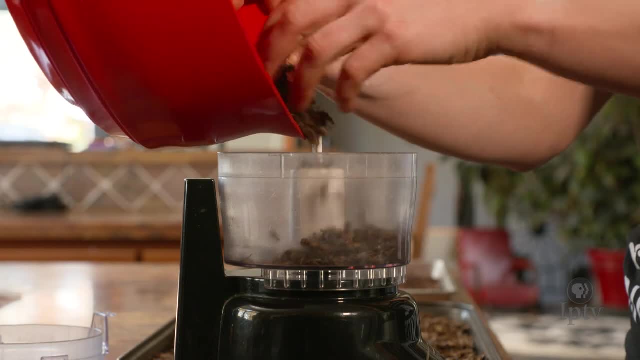 For every half-ounce pack there's about eight grams of protein. I get a lot of people that look at them and go, oh, it's got legs. My number one comeback for that is: well, do you eat chicken? I don't eat chicken wings. 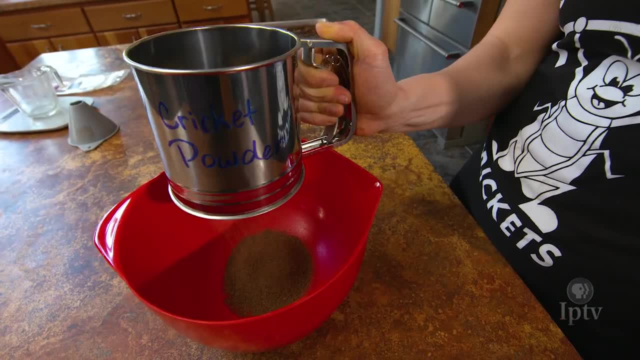 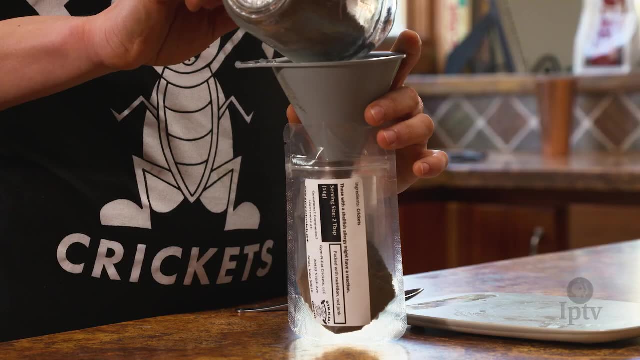 Now we're making sure all the scary stuff is gone, so all of the legs and the big bodies, it can be mixed into a protein bar or a smoothie or anything like that, Any baking recipe that you have chocolate chip, cookies or bread or anything like that. 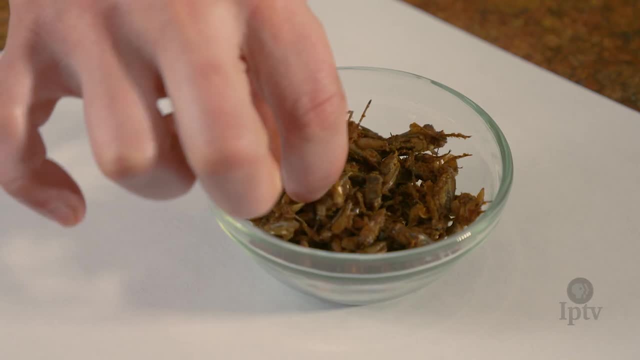 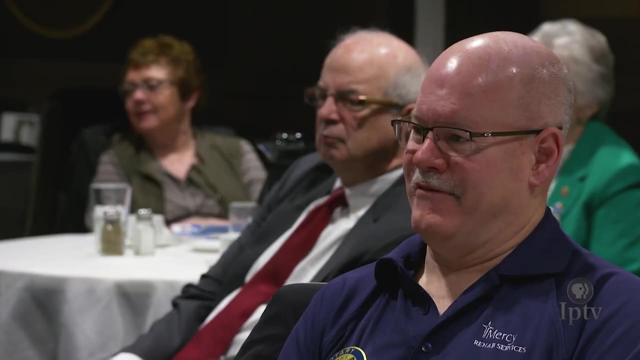 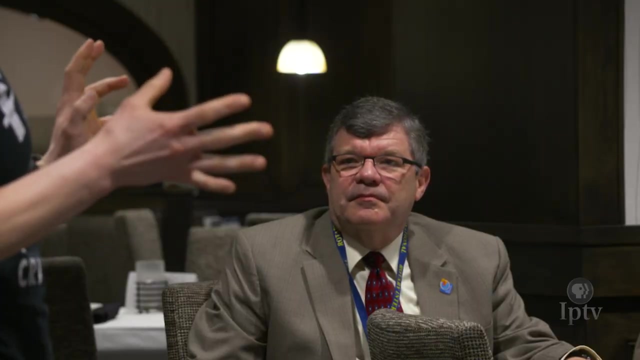 you can sub in a bit of cricket powder, So why would anyone want to eat crickets? Great question: Education is paramount. Education is paramount in what I do. Eighty percent of the world eats insects by choice. The population of the world is projected to be near 10 billion by 2050. 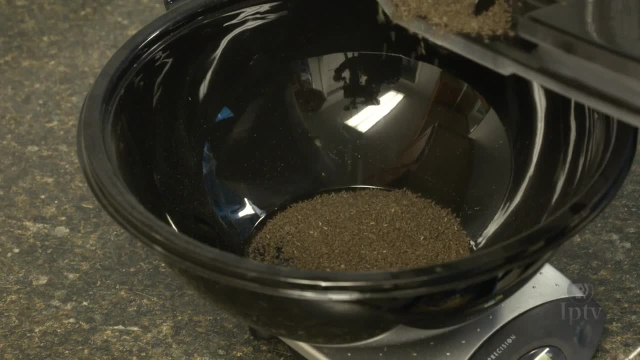 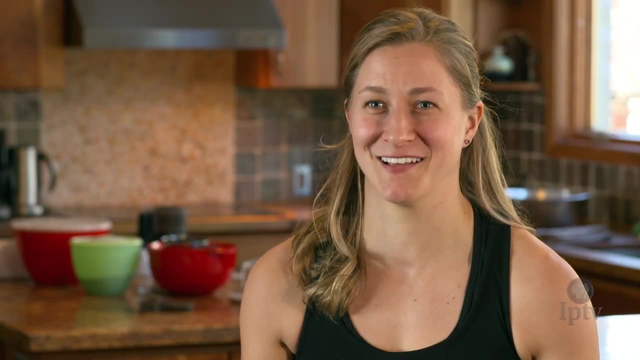 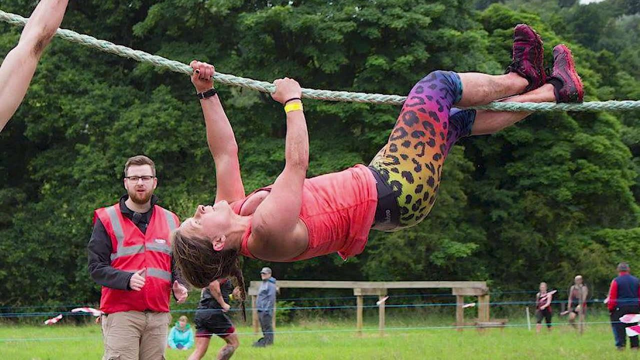 Current agricultural production is going to need to double. Where I go from here, who knows? because if you would have told me 18 months ago that I'd be raising bugs for human consumption- absolutely not. There is a carryover between being able to persevere 23 hours into a 25-and-a-half-hour 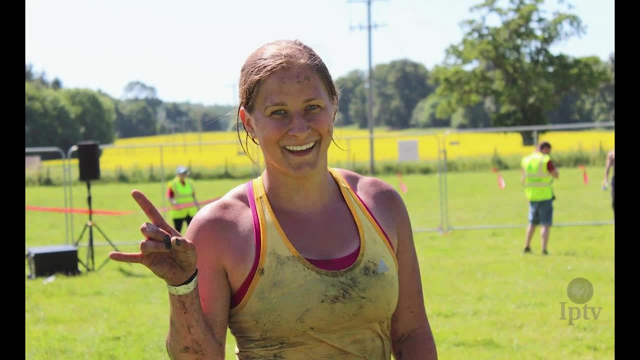 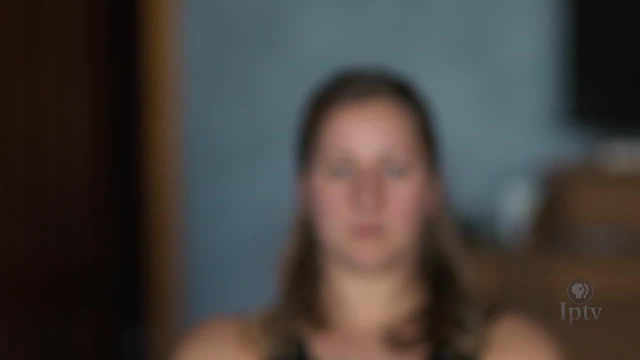 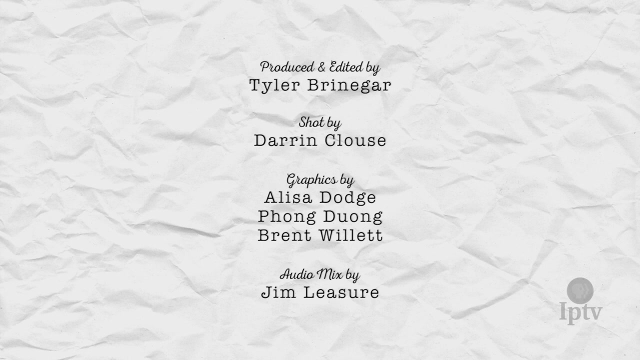 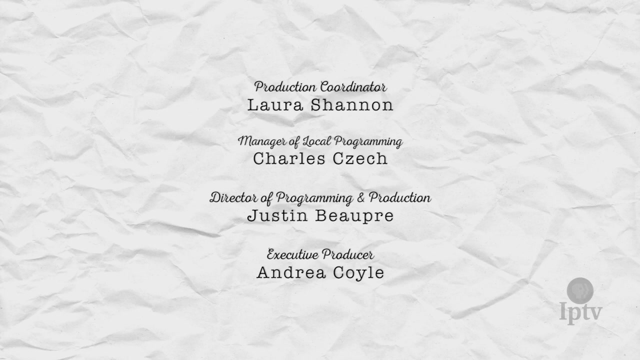 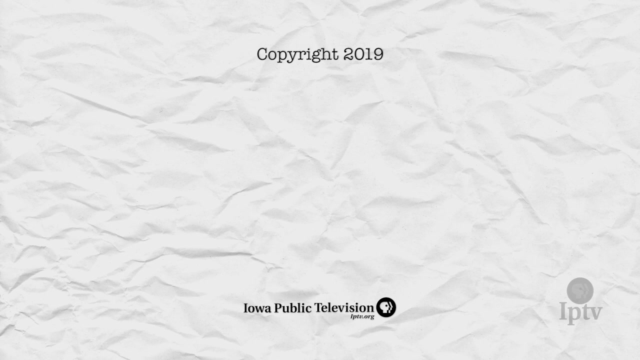 race and just keep moving and keep going. I actually prefer swimming at extreme, Bigger muscles that way. I actually hope this 없어요 is not high, but his back bend. I'd say I'd walk through that gate, Of course, Because I'd already had that in town at home. I definitely wouldn't cross that gate, Yeah.